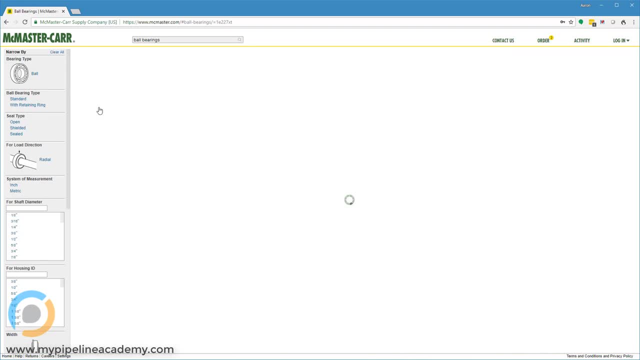 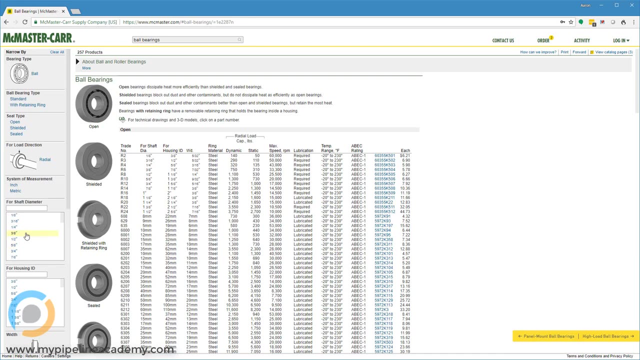 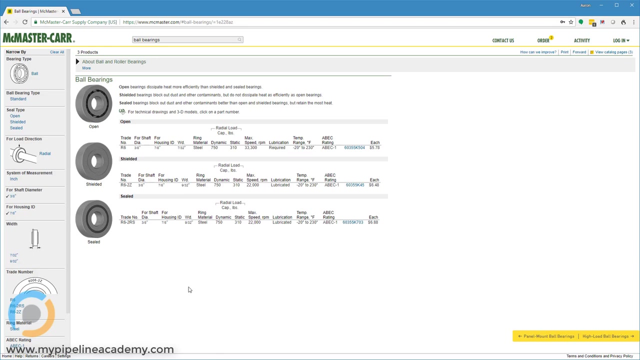 diameters are typically very high precision, In fact. let's just take a few. take a look at some of these here. We'll say, oh, I don't know, for shaft diameter three-eighths of an inch, And for housing ID seven-eighths of an inch. Looks like that's our only choice there. These: 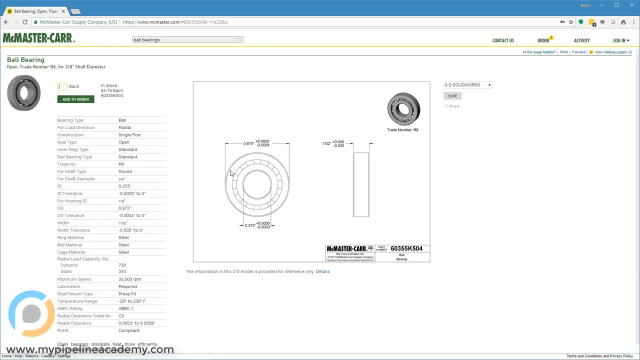 things. okay, And let's take a look at the drawing. Okay, so we have an OD of seven-eighths of an inch, plus zero, minus four-tenths For ten-thousandths of an inch. That's a. that's a pretty tight tolerance. And on the 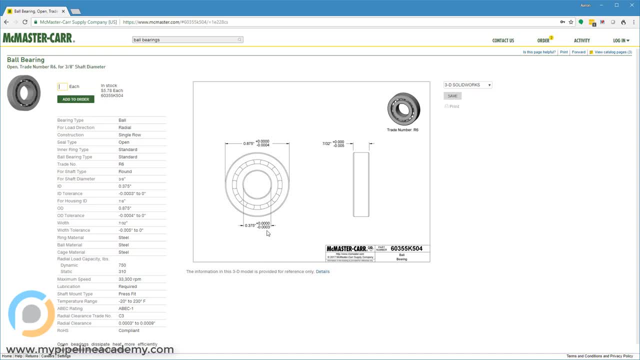 ID and the inner race, we have three-eighths of an inch plus nothing, minus three-ten-thousandths of an inch. The width is typically not as tightly toleranced, which is fine. That's not the critical geometry anyway. So you can see here in this one plus zero minus five. 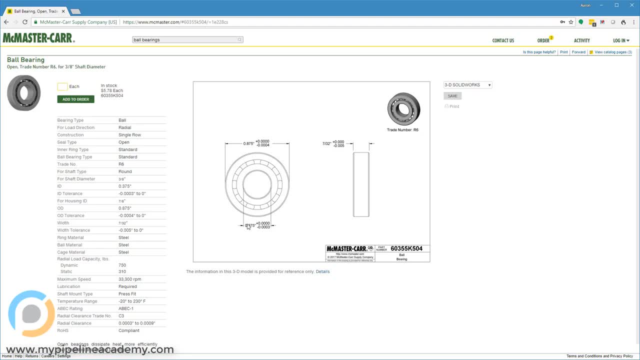 thousandths of an inch, Not ten-thousandths, Um, but uh, these, whenever you see, you know two, three, four, ten-thousandths of an inch and you see, if you can get one of these together you're going to Okay And so, but also, uh, basically, you just have to. 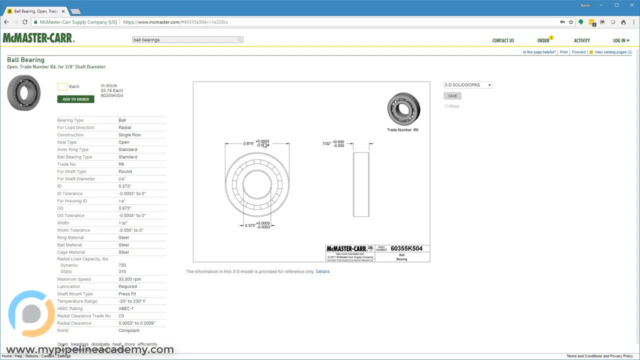 of an inch, you know that that's a good candidate for a press fit and in fact ball bearings are often press fit. the outer race will be: press fit into the block of whatever it goes into and then oftentimes you will press fit your shaft into the the inner race of the bearing. 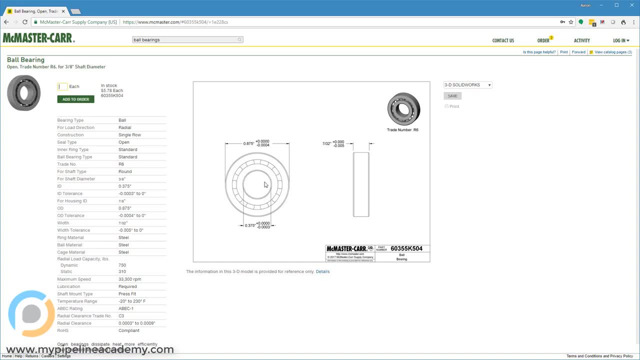 although sometimes it's. it's kind of more of a a slip, a tight slip fit or a transitional fit between the the axle, you know the shaft, and the inner race, but often it's a press fit with the outer race and it can be a press fit on the inner race as well. let's see. let's just look at. 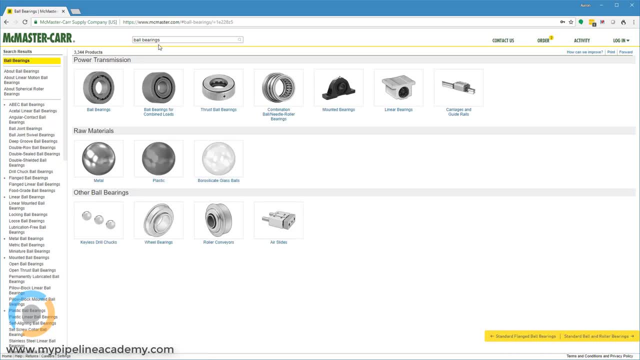 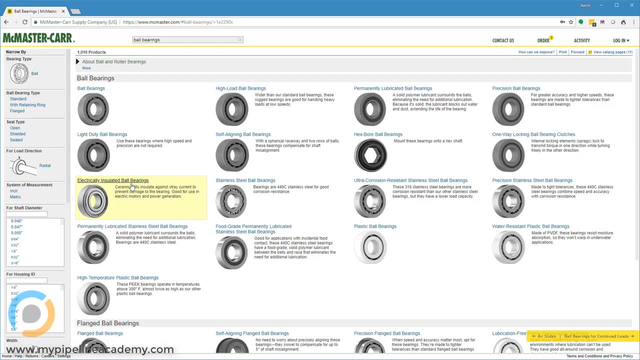 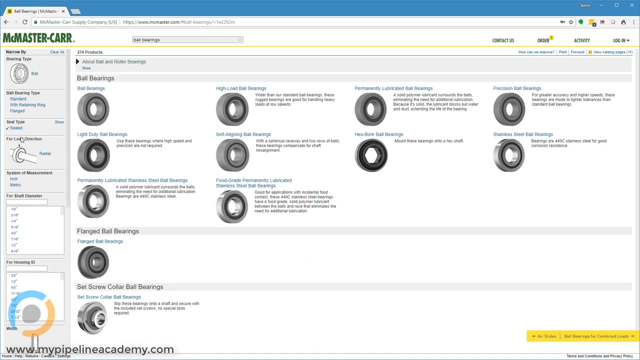 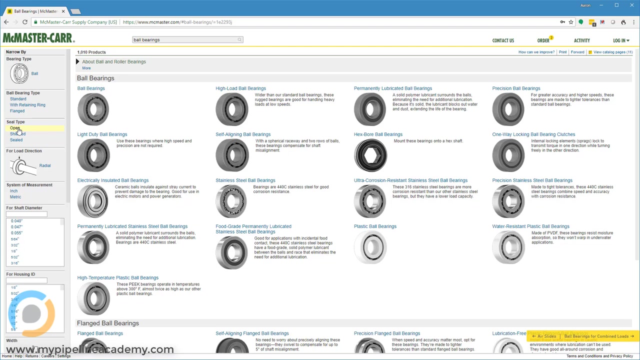 a few others, ball bearings we'll kind of look at. you know something pretty similar here, let's see. we'll say: sealed ball bearings come in a few different seal types. it can be open, which is the- uh, the least amount of friction, because there's there's no seal that um adds any resistance to that spinning motion. but the open. 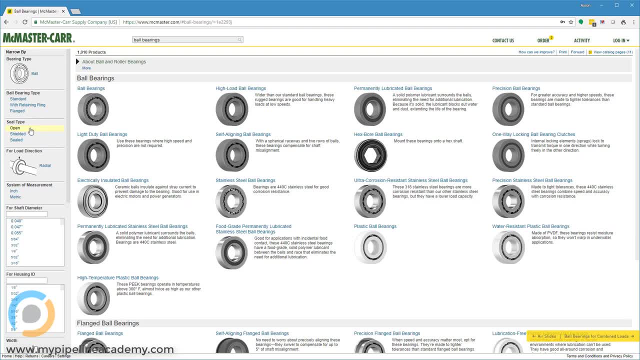 type: uh, you might get debris or some dirt might fall in there. so if you're working in a dirty environment or you know, maybe outdoors somewhere where it's dusty or something you you probably want at least a shielded or maybe ideally a sealed bearing you, and usually when you're working with ball bearings, a little bit of resistance is not going to be a big. 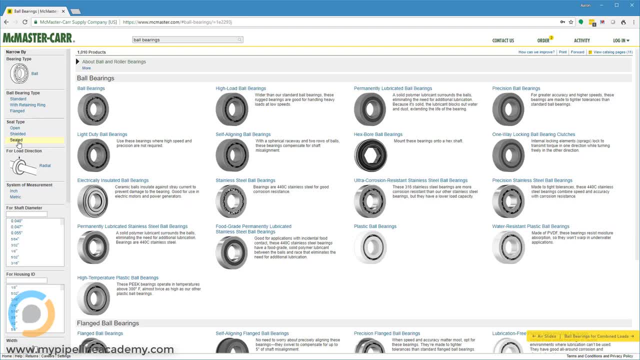 deal. um, if you're- i don't know- turning a motor shaft or something like that, a little bit of resistance is just not going to be a big deal. there are some applications where you want as close to zero resistance as possible, and for those i would suggest an open seal type which is no seal. 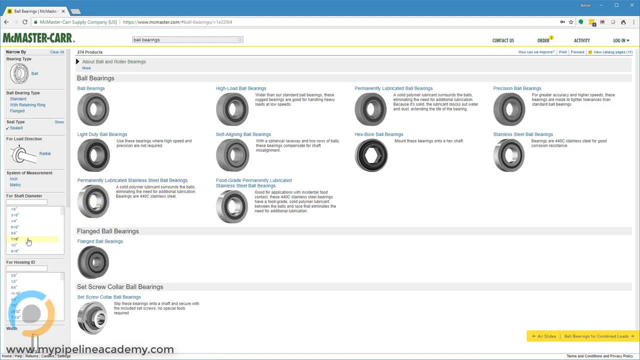 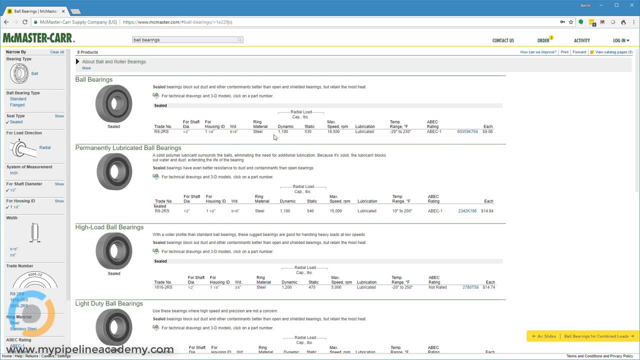 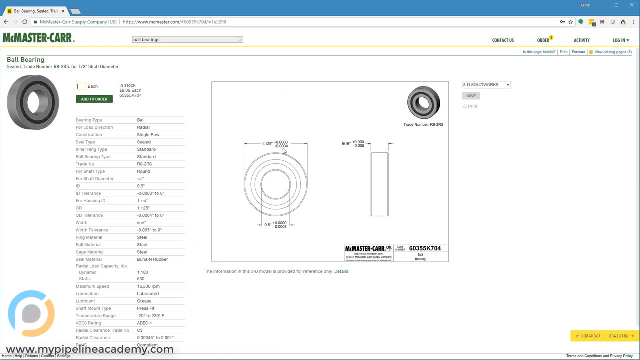 um, so let's see. i don't know if we looked at a sealed one and maybe this thing will say: for a half inch diameter, uh, shaft, and one and an eighth, i don't know, let's select this one and see what that looks like. all right, so almost identical. in fact, i think they are the same tolerances here, plus mine. 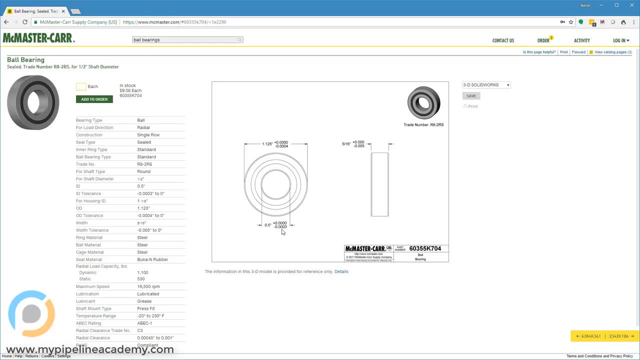 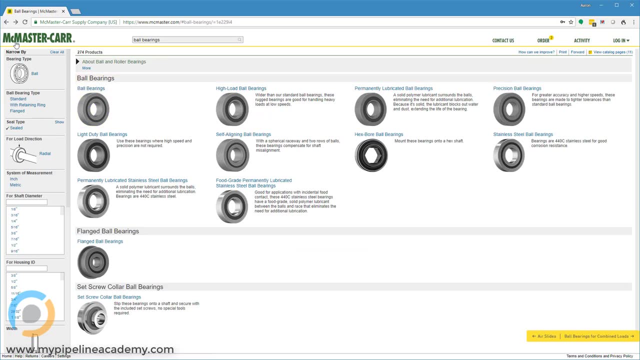 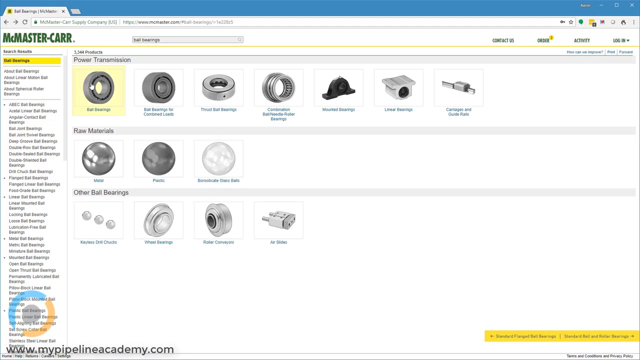 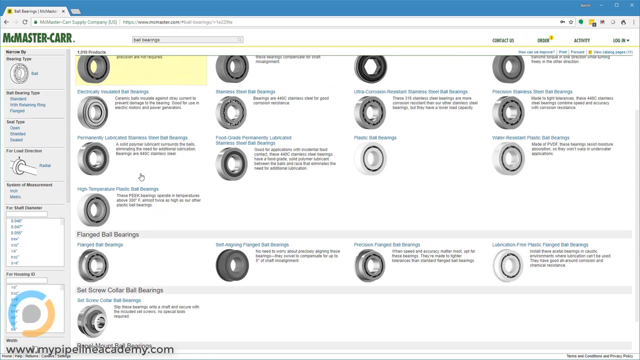 plus nothing minus four tenths on the outer race, plus nothing minus three tenths on the inner race. well, let's go back a little, a few pages here and see what else we can look at. okay, something else i wanted to to show everyone is: uh, there are what are called needle roller. 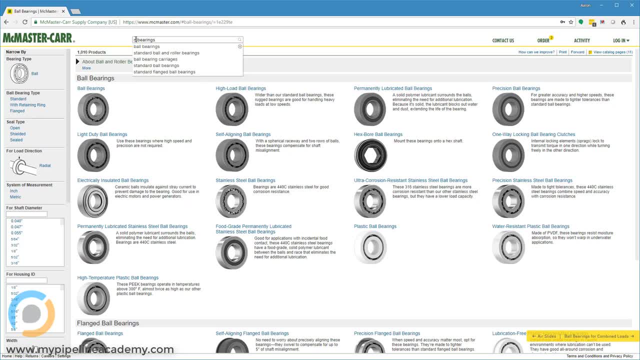 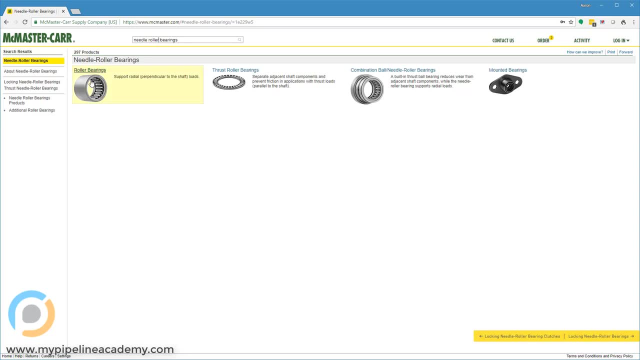 bearings. let's see needle roller bearings, and instead of small steel balls, these needle roller bearings have, um, they're almost like really small dowel pins inside the detail, but um, there's also a Audioёмity making a ring and going to. you know, the Fu primate thing. i've never had a forward rollerStravata. 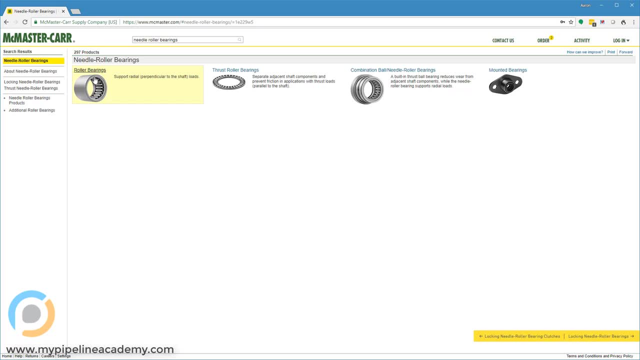 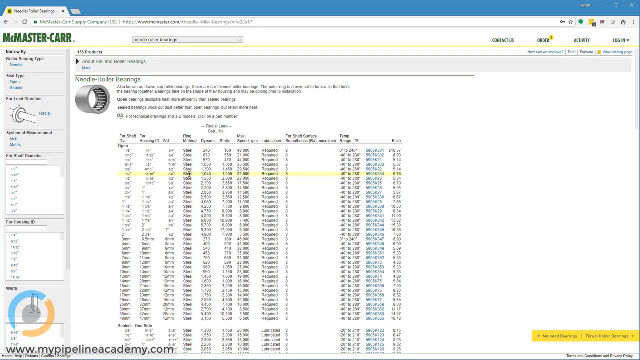 so they don't. !40% less weight when hundred way kinds like right now, and i don't think they shiny. all right, and let'sMusik inside there that replace the balls in ball bearings, And these needle roller bearings typically have a higher load capacity. 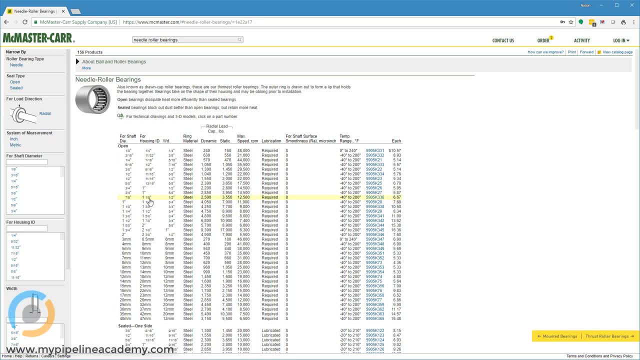 So let's see, this one is for I don't know. let's compare apples to apples and say: let's look at a quarter inch shaft diameter. So this one right here rated at 570 pounds for dynamic load And if we go to a ball bearing, that's a quarter inch. 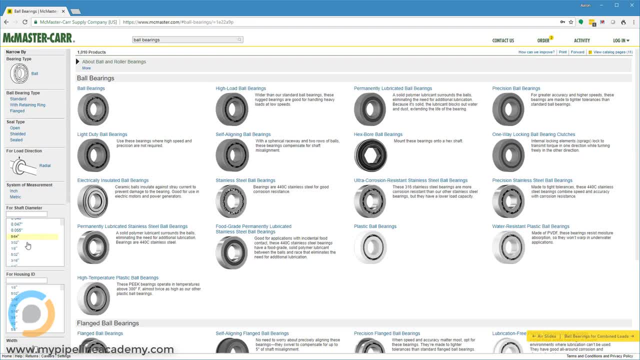 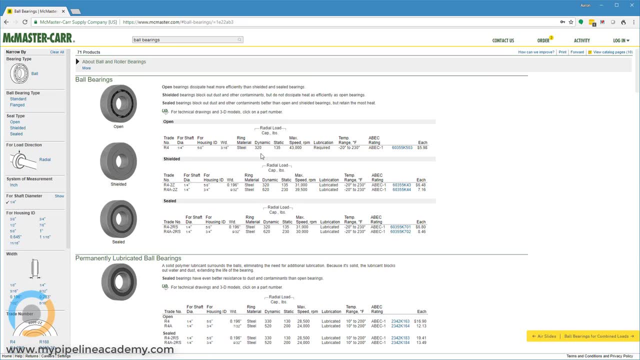 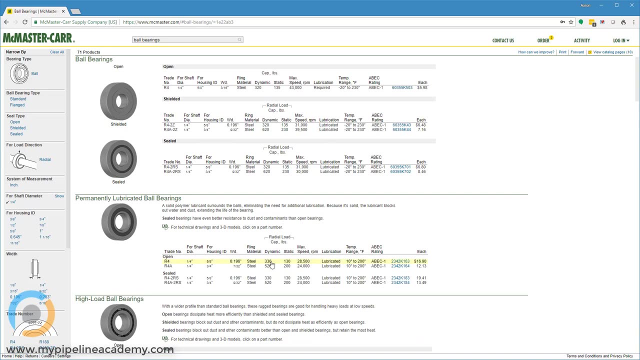 for a quarter inch shaft, that is for shaft diameter, quarter inch. our load capacity is 320 on this one, 320 on this one. This one's pretty high actually: 620, 320, 620.. Down here we've got 330, 520, 330, 520. 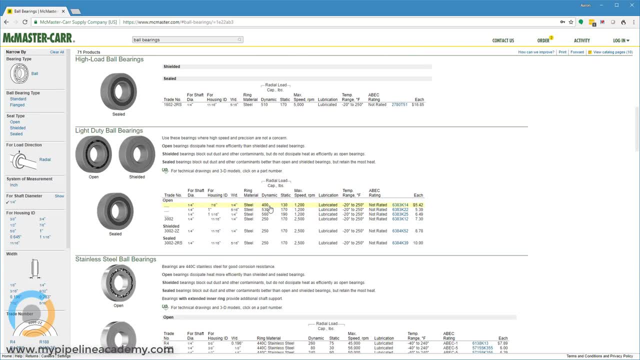 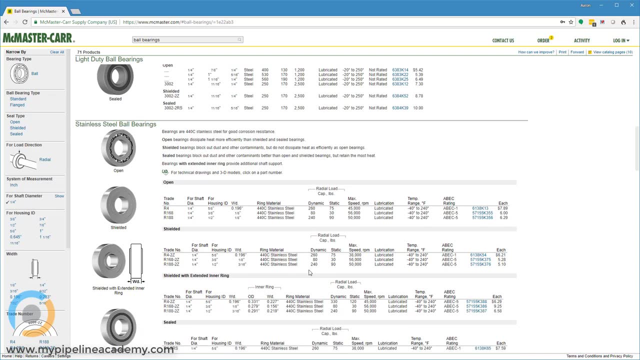 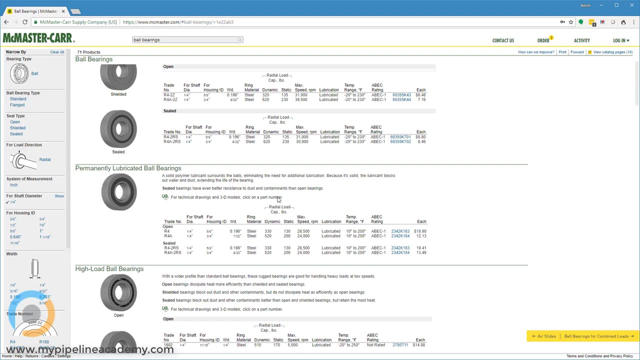 So generally a little bit lower, A few more down here: 400, 250, 250,, 260,, 80, 240.. So anyway, needle roller bearings offer a little bit higher load capacity, Let's see oftentimes. oh, let's look at one other thing. 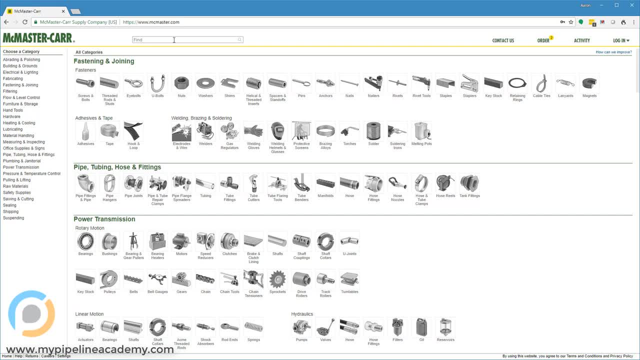 So ball bearings and needle roller bearings, they're not terribly expensive. You might pay, I don't know, $5 or $10, maybe a little bit more for one of these, But if you're using an application where cost is a factor and you're, 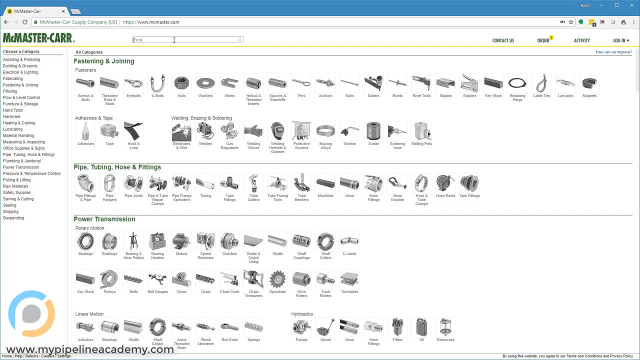 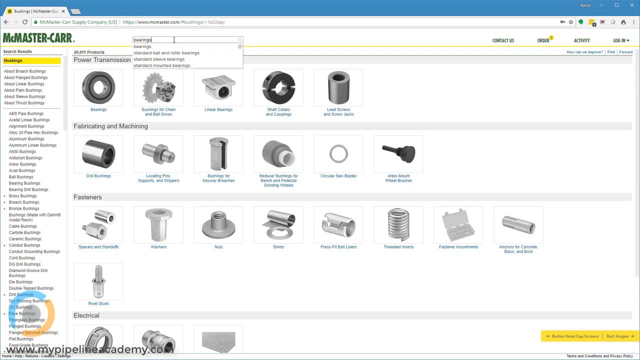 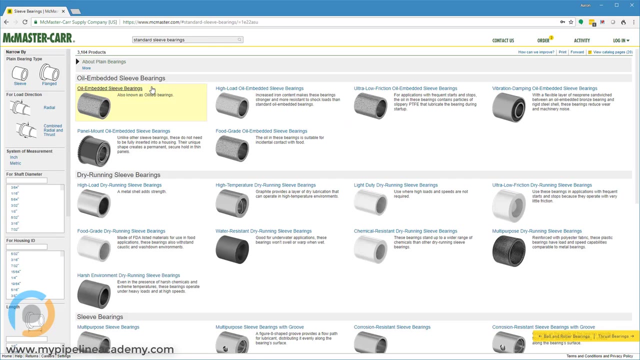 trying to get really low cost bearings, you can use what's called a sleeve bearing. So here's an example of a sleeve bearing, And a sleeve bearing is basically just a cylinder. It's a cylinder made out of a low friction material such as oil embedded brass like this one right here often. 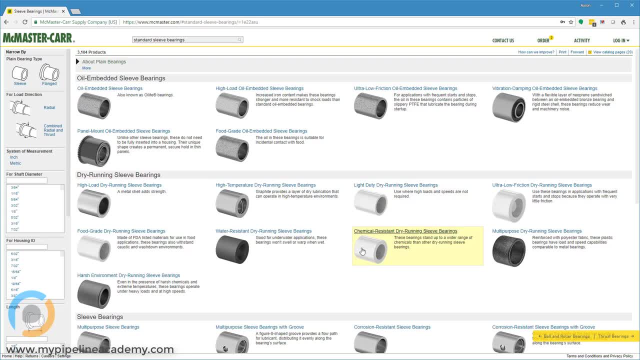 referred to as oil light bushings, There are also plastic ones. Let's see what plastics do they have here. Material: I saw nylon, UHMW, acetyl, PTFE. These are all really low friction plastics And again they're just a cylinder. 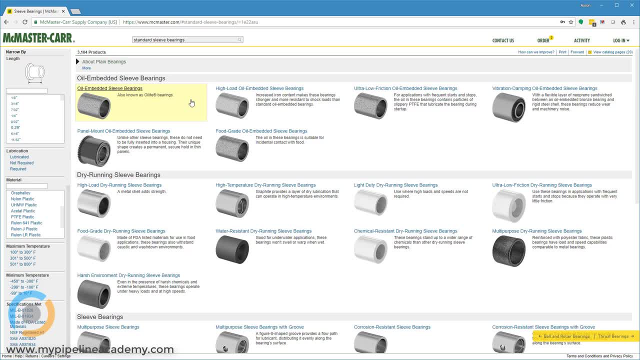 There are no moving parts in them, no balls, no needle rollers, just a plain cylinder and that's it. And they're not as high precision, They're not as smooth, as low friction as ball bearings are, But they're certainly cheaper. 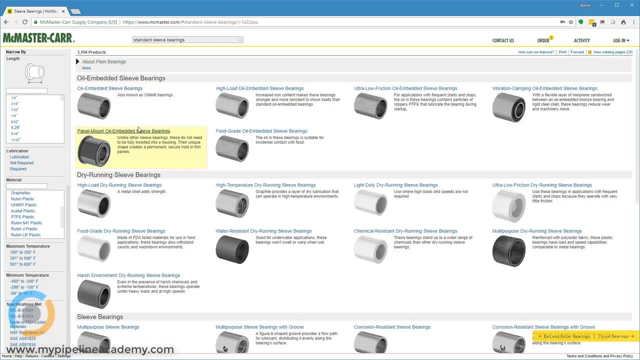 You might pay- I don't know- $0.50 to a couple of dollars for one of these sleeve bearings versus a ball bearing. So that's an overview on what some of these bearings are. Next we'll take a look at what a real world design looks. 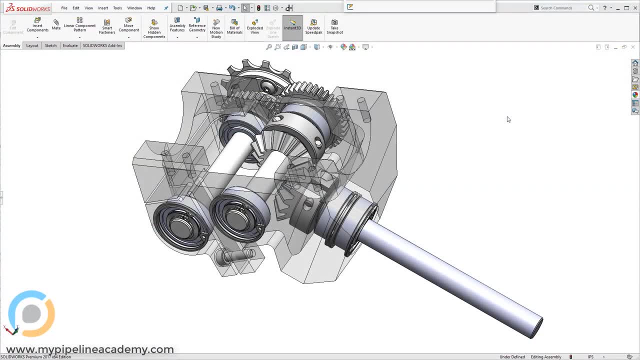 like: Let's take a look at what a real world design looks like. So let's take a look at what a real world design looks like. So this is a real world design. It's a real world design that incorporates some ball bearings. 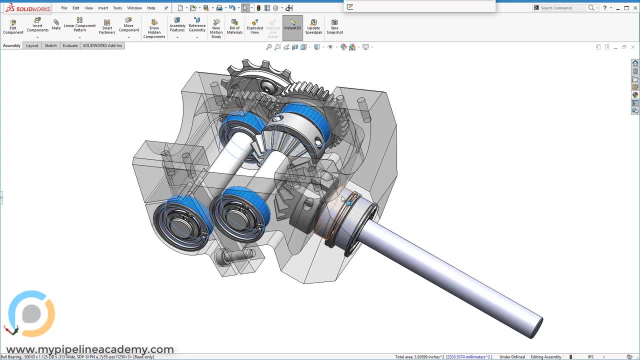 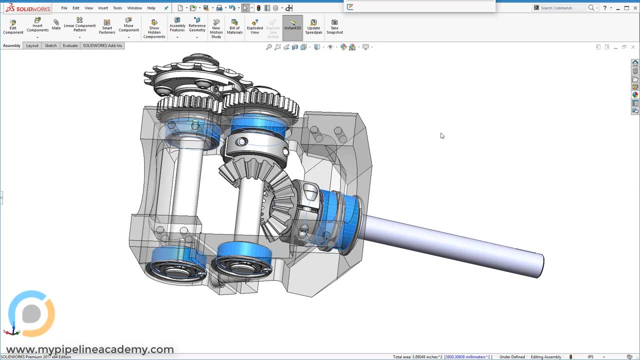 Here's a gear train or a gearbox that we designed a few years back. You can see right here there's a ball bearing. This is another one there, another one there and there and two more here, And if you look at how many axles are in this, 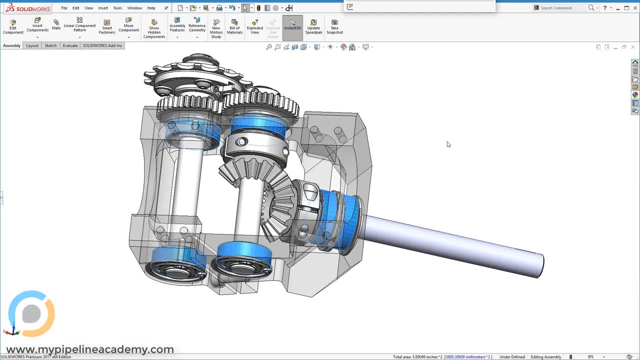 you can see that there are a number of bearings associated with each axle, And that's the ideal way to incorporate bearings when they're used with axles, Because having a bearing on either side of the axle or, in this case, we weren't able to get a bearing. 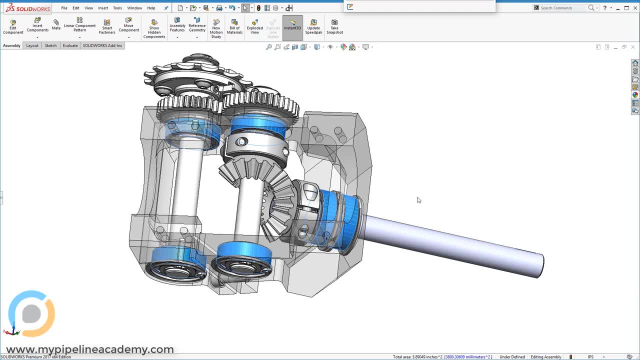 on either side of the axle, but we did have two bearings next to each other And that just provides better support for your axle when it turns, better stability for rotation. So that's a best practice, whenever you can, is to put a bearing on either side of your axle. 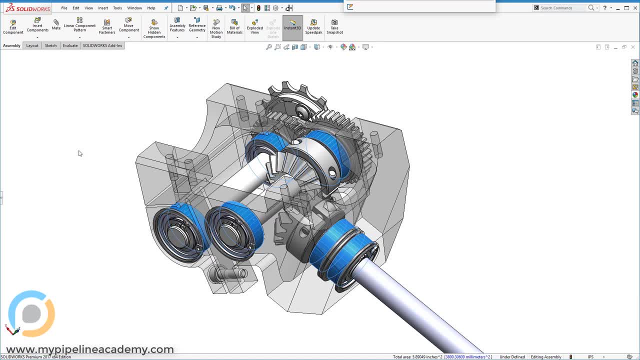 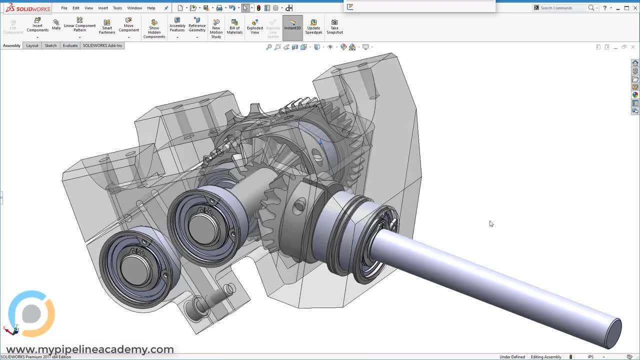 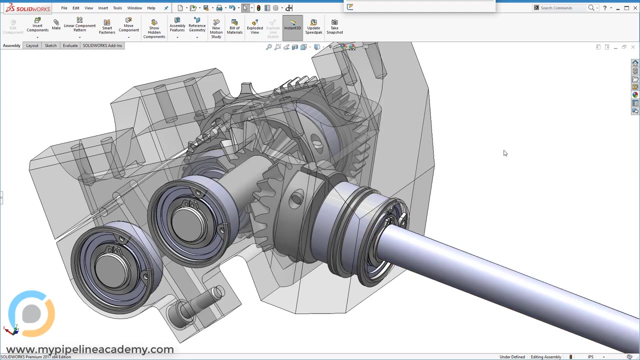 And then something else I'll point out, and this is a common way to hold bearings in place. I mentioned earlier that bearings are often press fit in place And that was the case in this design, But we wanted kind of a backup assurance that these bearings wouldn't come out. 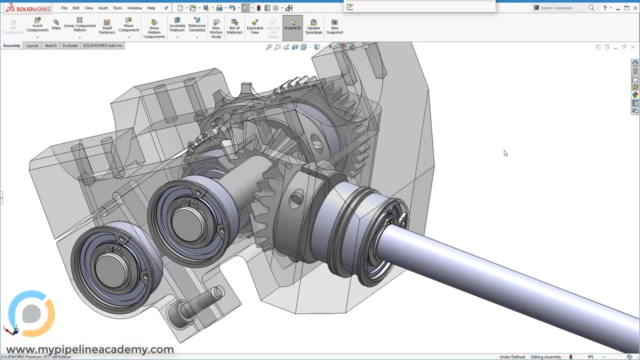 Maybe it gets really, really hot one day out in the sun and the material, this block of material, which was aluminum, expands a little bit And these bearings start to lose their press fit. Well, we put these retainer rings in here. 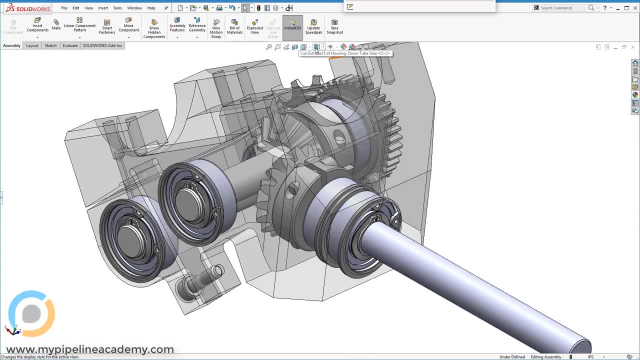 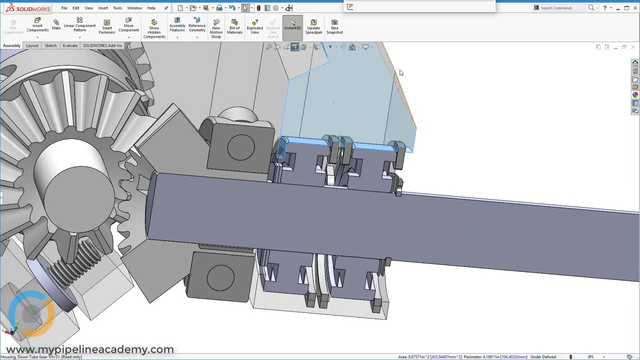 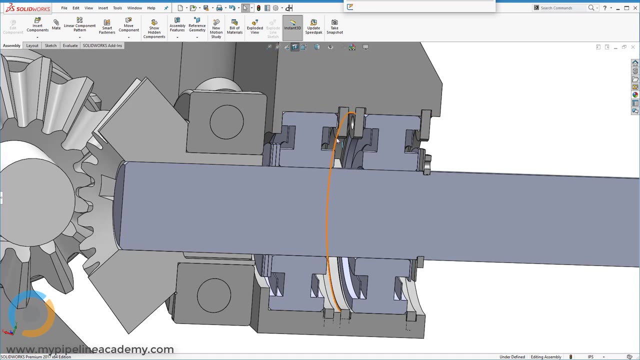 These guys right here. Let's see if I can do a cross section. There we go. That's a good view, And I'll make this opaque. There we go. We can see these grooves that were cut into the aluminum And then these retainer rings that were placed. 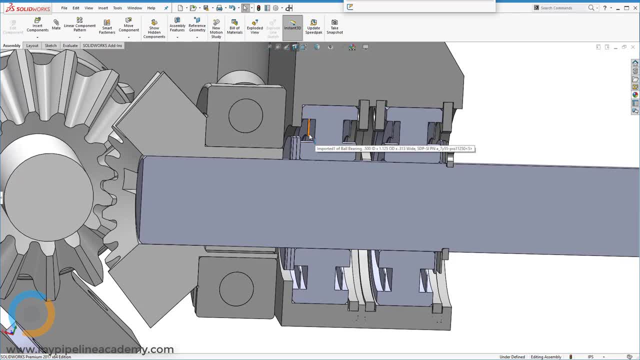 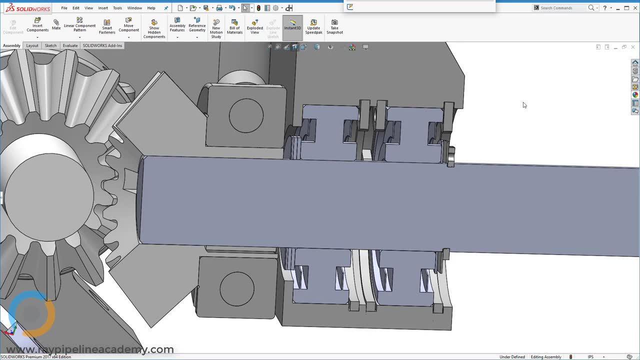 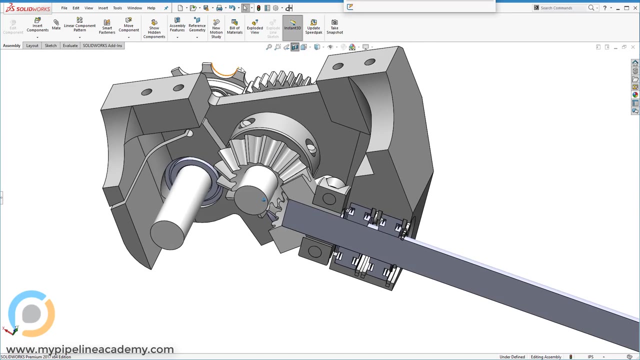 in those grooves And those retainer rings. just keep these bearings in place, And that's a common method of holding a bearing in place. whether it's a ball bearing or a sleeve bearing, Either one would work just fine. What else can we look at here? 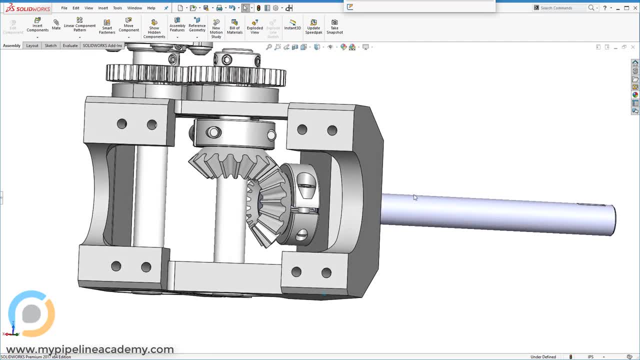 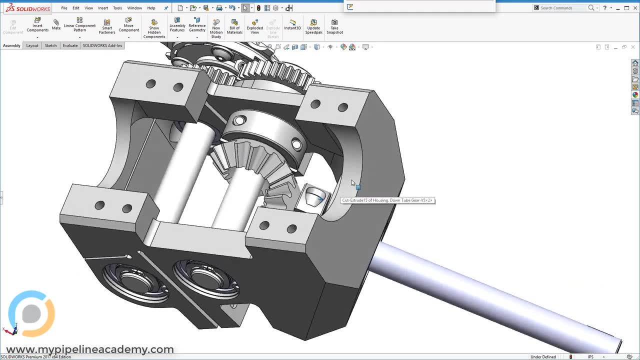 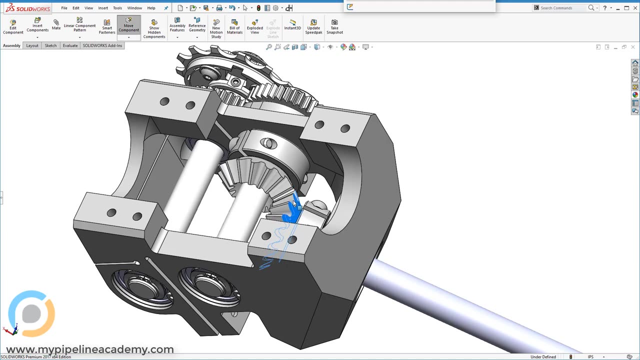 It was very important in this gearbox that we have extremely, extremely precise positioning between our two bevel gears here. In fact, I'll kind of spin these around a little bit so we can see There we go, How everything moves together. But when you're working with gears, 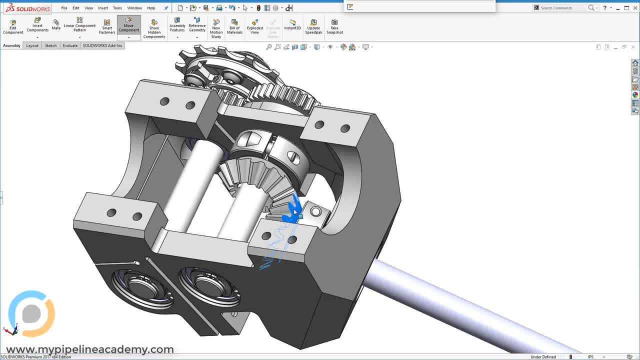 it's critical that the relative positioning between the gears is very, very precise. Otherwise, your gears won't be as efficient, They'll wear out more quickly, And so you want the positioning of your gears to be within a few thousands of an inch. 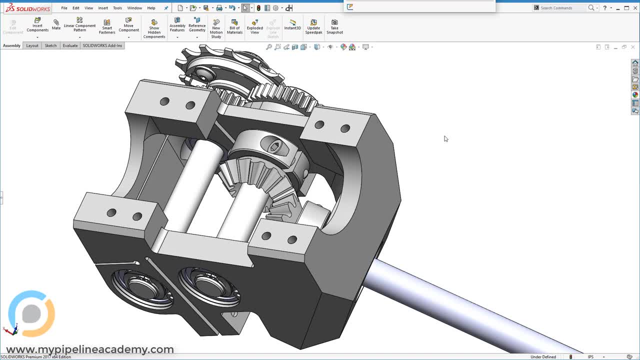 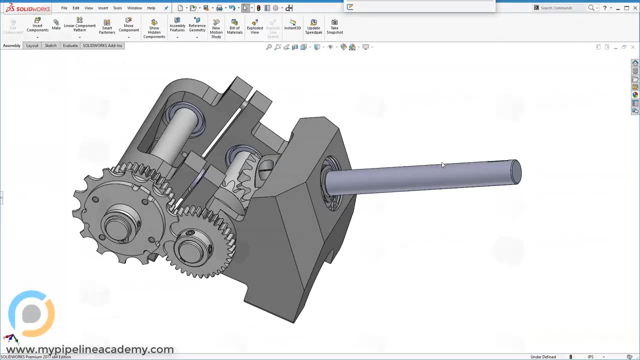 of nominal positions And ball bearings because they are very high. high-precision pieces of hardware allow you to do that, And that's another reason that we, another reason why we used ball bearings in this application. Another type of ball bearings I want to look at. 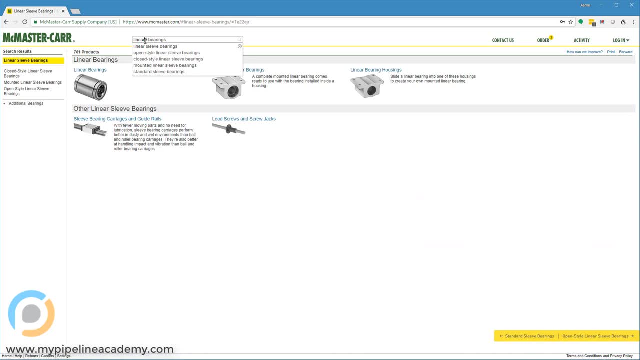 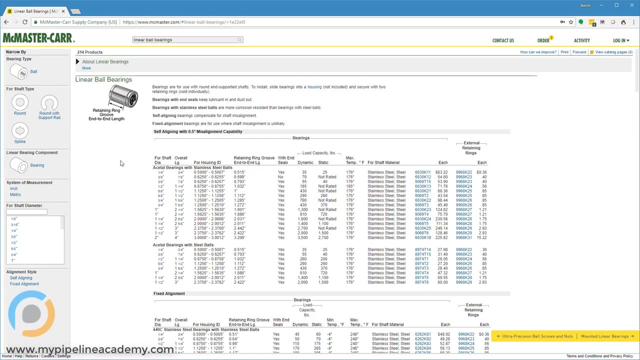 are linear ball bearings. Linear ball bearings And, as the name implies, linear ball bearings allow you to move something linearly very smoothly. There's kind of a serpentine. you can't really see it very well in the picture, but you can see a little bit of it. 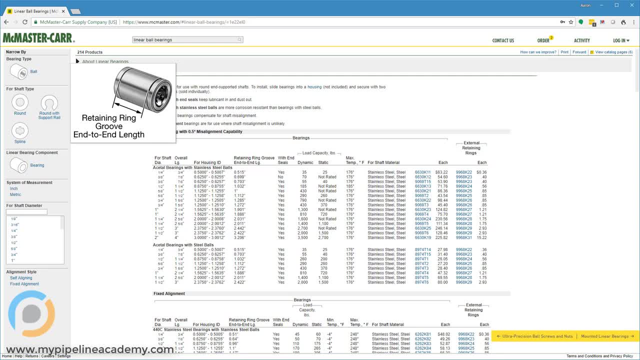 right here at the end There's kind of this like serpentine back and forth racetrack pattern of little tiny balls inside these linear ball bearings, And so your shaft runs through the the inside of the linear ball bearing where sometimes your shaft is stationary. 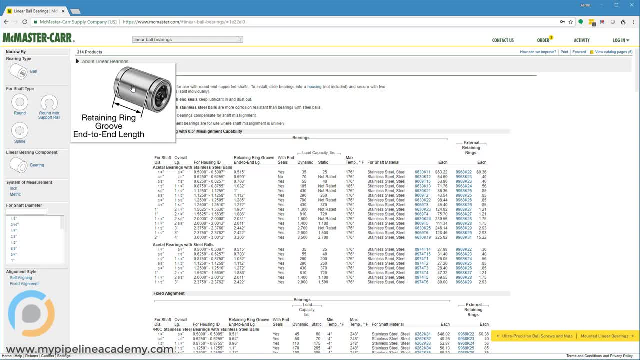 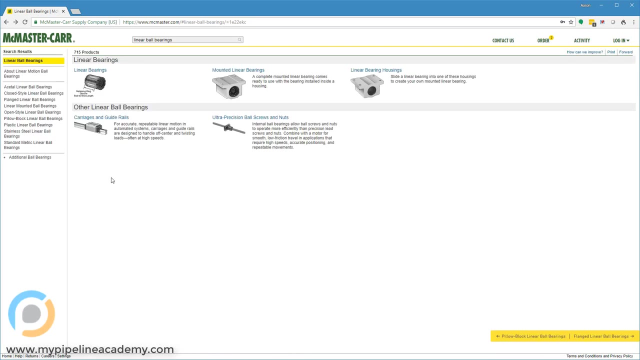 and the linear ball bearing runs on the outs is what moves on the outside of your shaft. But whereas typical ball bearings will allow something to spin very smoothly, these bearings allow something to slide back and forth very smoothly, And there are a few different types. 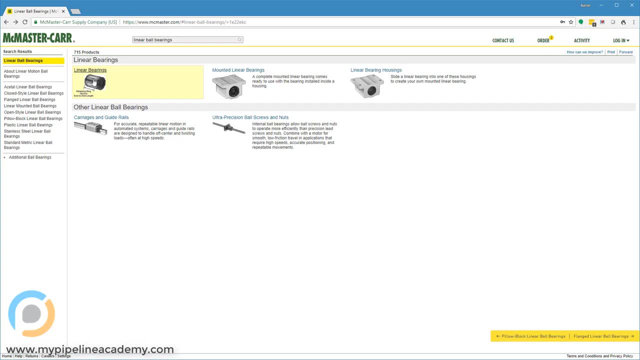 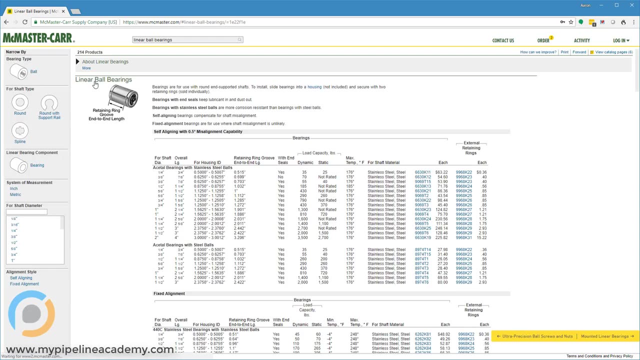 so these linear ball bearings that we were just looking at you can incorporate, you know, into anything you want. You just drill a big bore out of your material and you can press fit these linear ball bearings in place, or, more often than not, 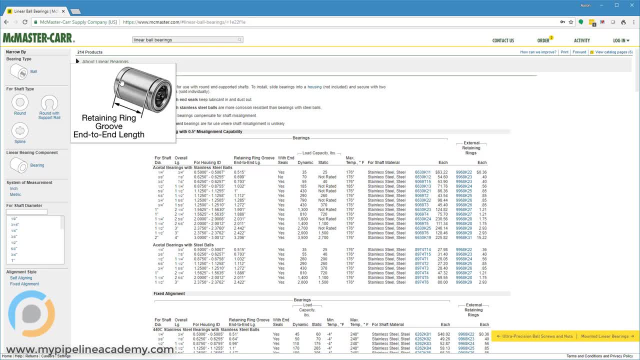 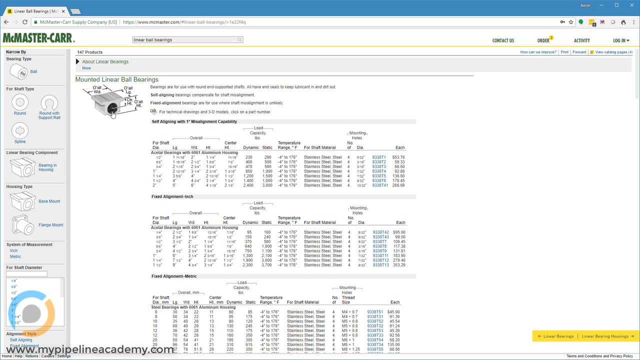 you use these little retaining ring grooves to lock them in place. You can also buy them already incorporated into blocks of material, something like this: And then you- just you know- screw these the enclosure holes onto whatever you're using with. 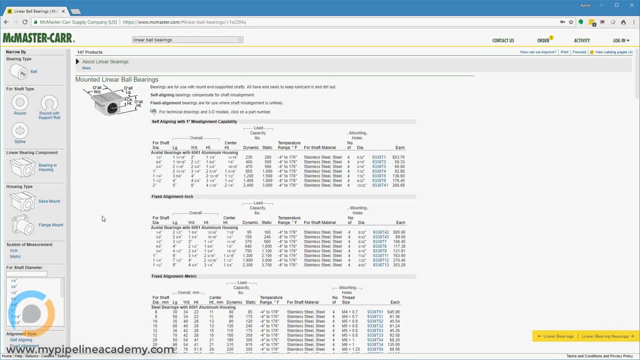 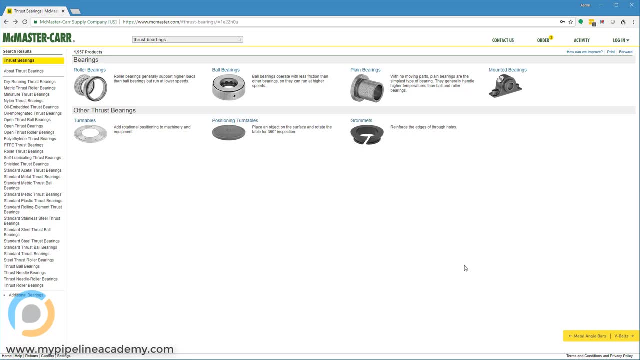 So those are linear ball bearings. Finally, the last type of bearing that we'll look at is what's called a thrust bearing, And there are a few different types of this kind of bearing. Sometimes the simpler, less expensive versions are called thrust washers. 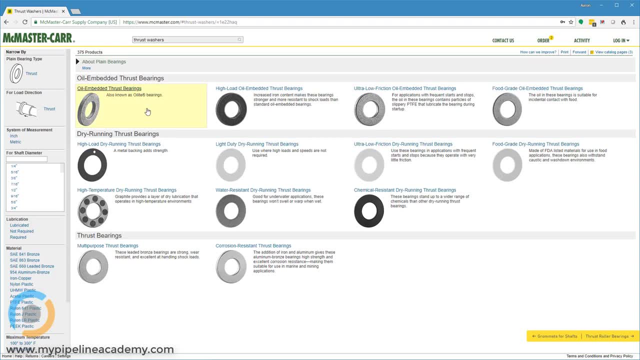 And a thrust washer is basically just a disk of material, kind of like a sleeve bearing is just a cylinder with no moving parts. A thrust washer is just, you know, just a disk and it's made out of a low-friction material. 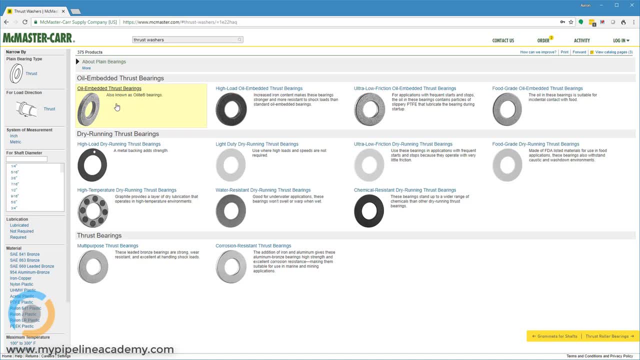 We have this oil light material again, that oil-infused bronze. Down here we've got bronze with graphite powder embedded in it. Some of these are plastic. We probably have some UHMW, some PTFE, maybe some acetyl. 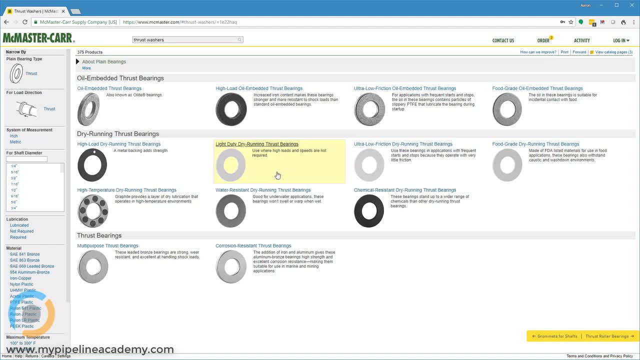 Those are all very low-friction plastic versions. So thrust washers And thrust washers are used when, instead of something, instead of a load, being placed in the radial direction, when something is spinning, as would be the case with a ball bearing. 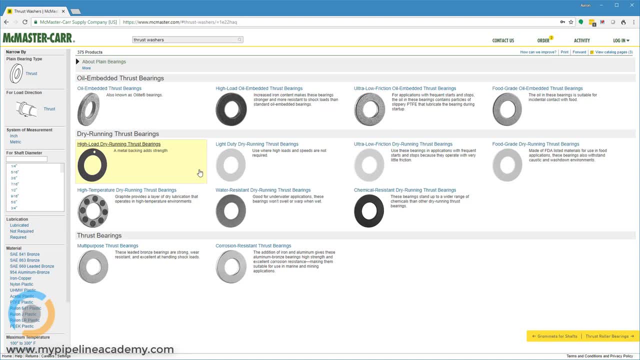 for thrust bearings you have again. you're working with a rotational motion, but the load in this application is in the axial direction instead of the radial direction, So the load would be placed on the face of these bearings, kind of where I'm pointing right here. 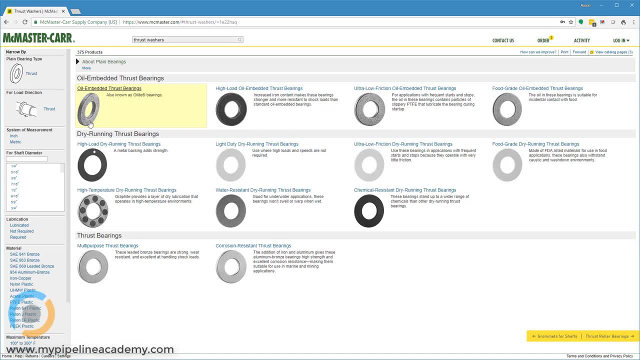 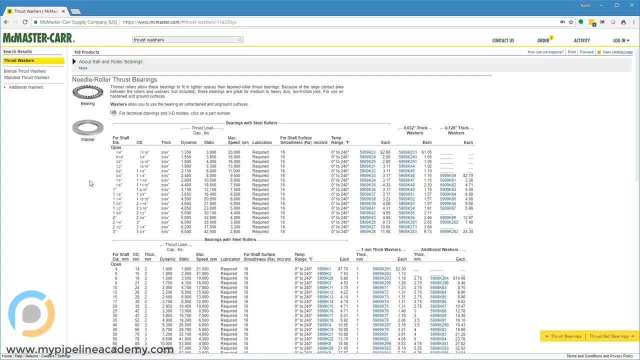 If you pushed on that face and turned, that's the kind of application for which you would want to use a thrust washer or a thrust bearing. So going back here, another type is thrust roller bearings, And just like the needle roller bearings, we also have needle roller thrust bearings.